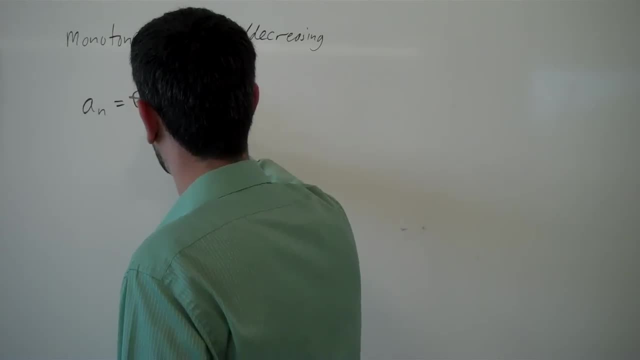 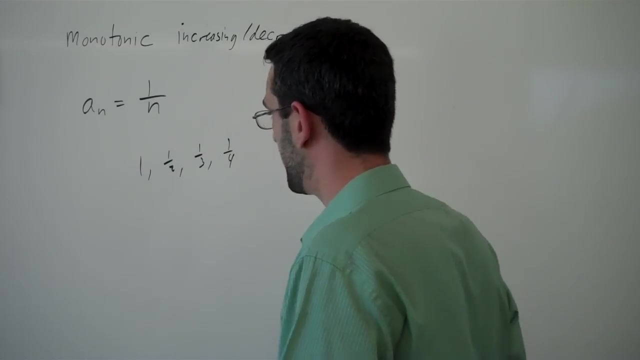 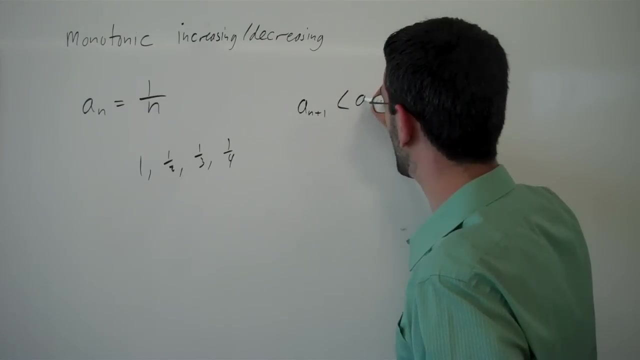 for example, if I looked at this sequence and we start listing out a few terms- one, a half, a third, a fourth- you'll notice that these are always getting smaller, right? In other words, a n plus 1 is always less than a n, And so this we would call. 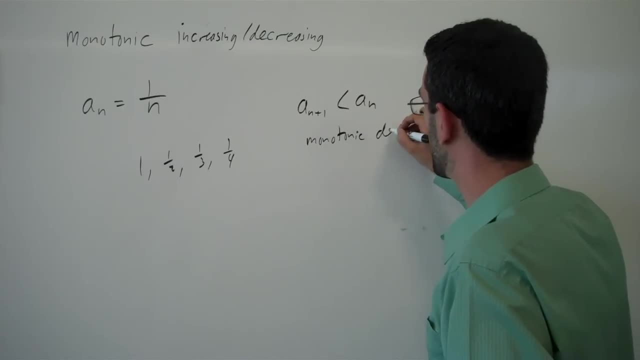 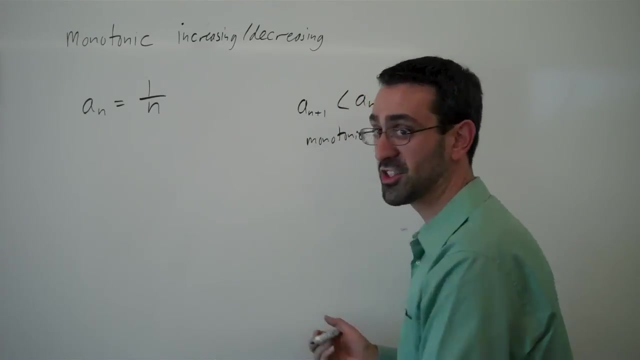 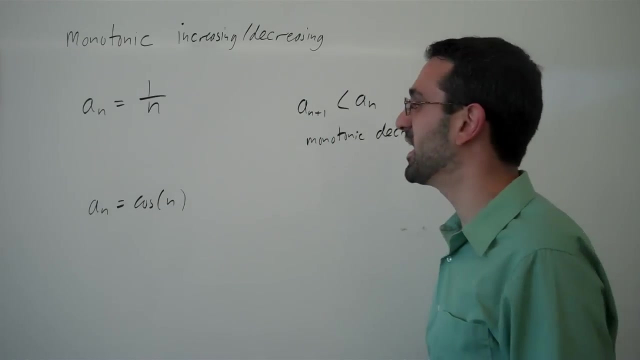 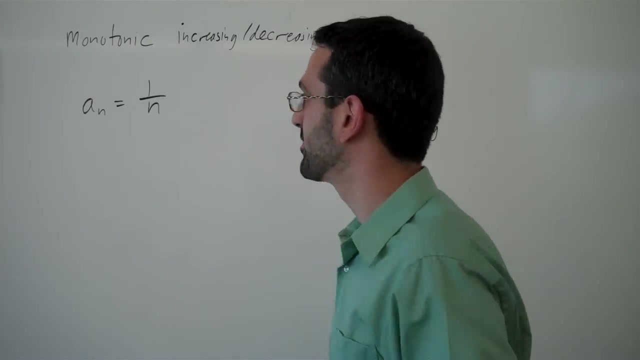 monotonic decreasing. Now you can compare and that to sort of an extreme example, something like a n equals cosine of n, which is going to oscillate up and down. this is certainly not monotonic. increasing or decreasing, it's neither okay. so that's the idea of monotonic. so then, the other concept we're going to talk about is the 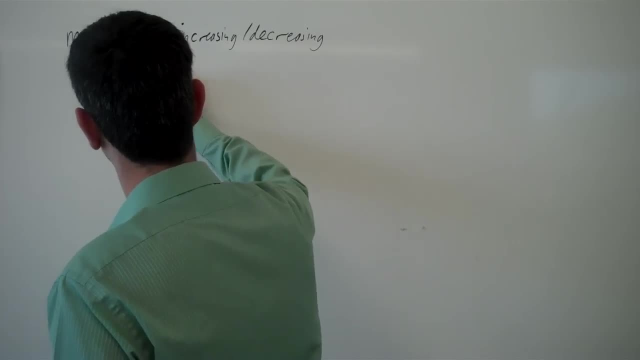 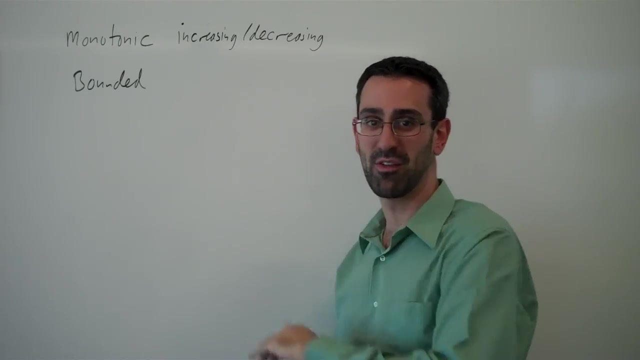 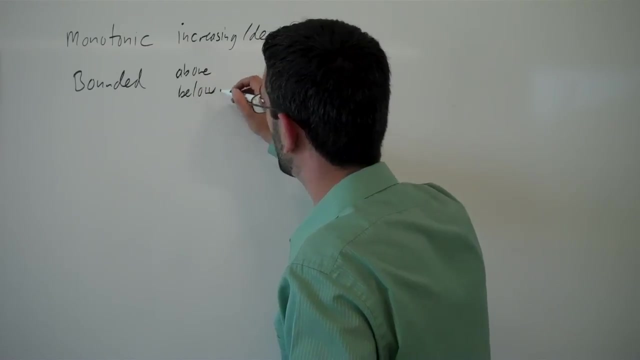 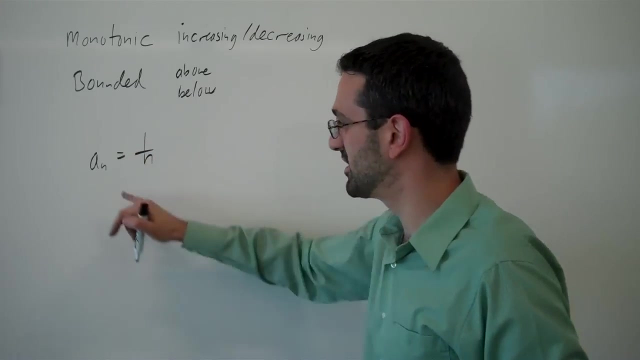 idea of bounded. so a sequence is bounded if there is some value that it never gets higher than, or some value it never gets lower than. that's either bounded above or bounded below. so for example, again an equals 1 over n. notice that if n, since n is always a whole number, since n is always positive. 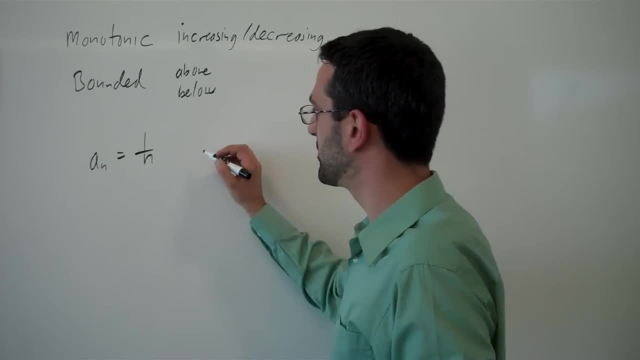 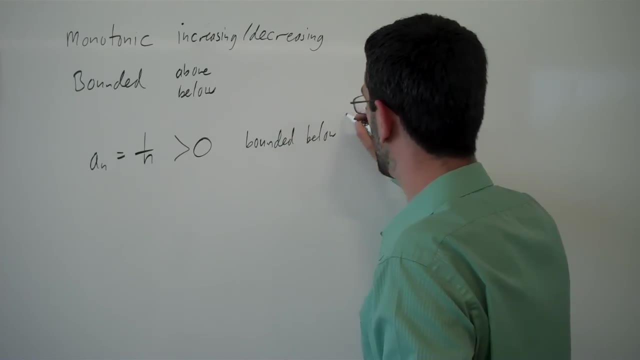 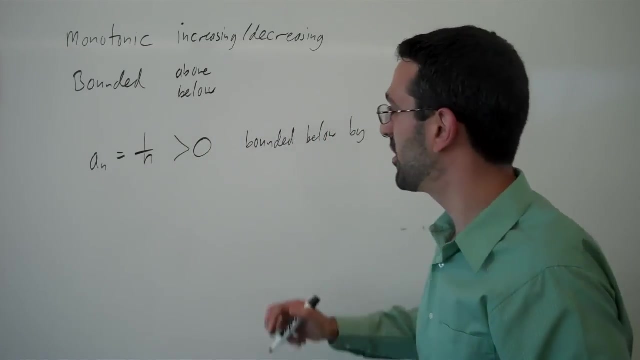 1 over n will always be a whole number, and since n is always a positive one over n will always be a whole number- positive- this is always greater than zero, and so that this is bounded below by 0. now we also know that this is decreasing, which means it's always getting smaller, so it's also bounded above by. 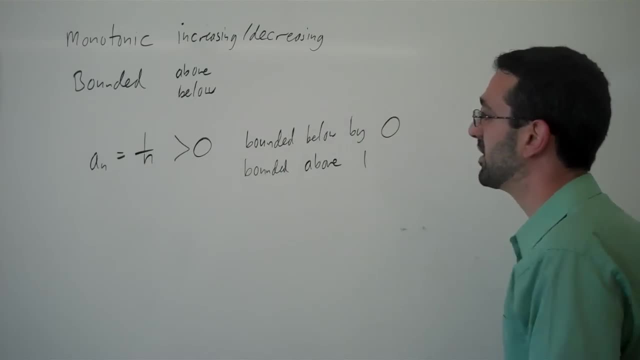 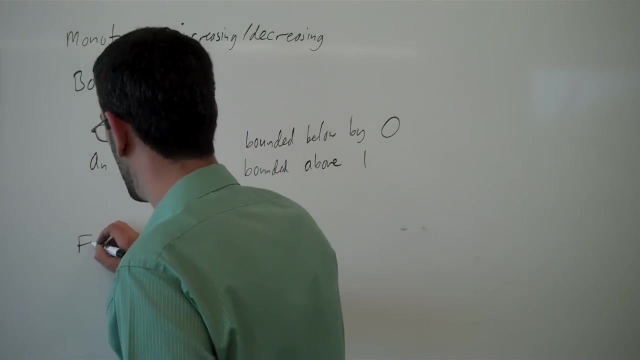 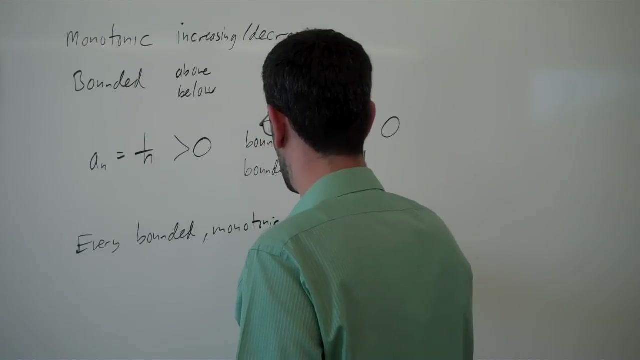 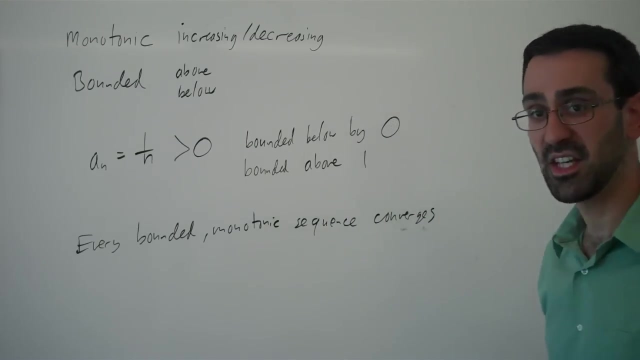 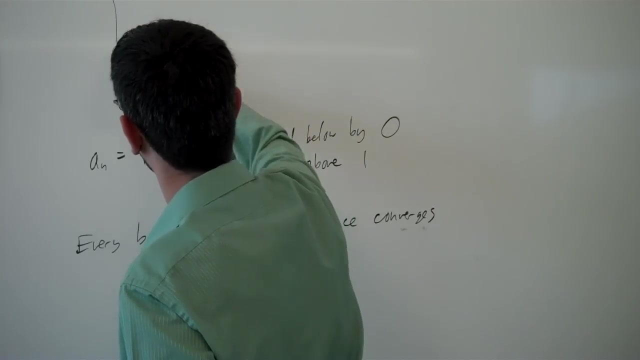 whatever the starting value is- in this case it's 1, alright, so this sequence is both bounded above and below, And there is a theorem which says that every bounded monotonic sequence converges. And let's think about why. So imagine we have a sequence of values and we know that those values never get smaller.